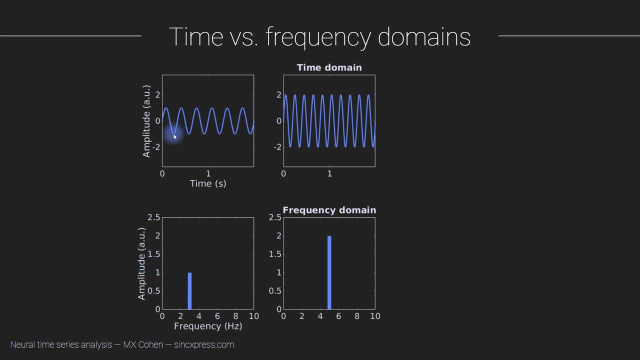 and that corresponds to one half of the distance between the troughs and the peaks. So you can see. well, I guess you can't really see, but there's no tick here. but you can imagine that this is minus one and this is plus one. So the 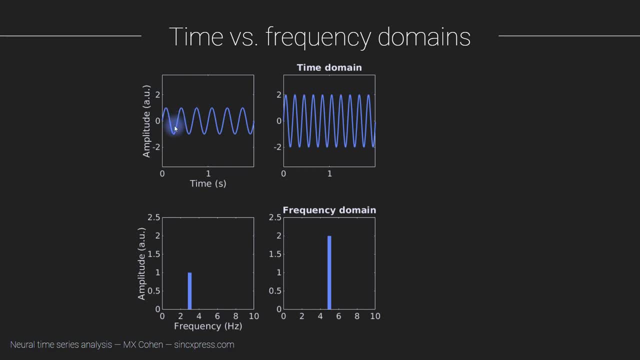 distance from the trough to the peak is actually two, because we go from minus one to plus one, and so one half of that distance is the height that gets plotted here. Now, why that is one half of the distance and not the full distance is an gluten binary now, but it will make sense in a few videos from now when we 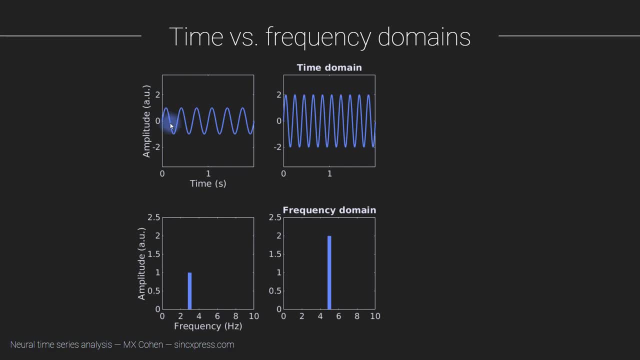 start talking about complex sine waves and complex dot products. So for now, suffice it to say that the amplitude value here corresponds to half of this distance. All right, so let's do the same procedure for this signal here. So we have one, two, three, four, five cycles within a period of one second, and then 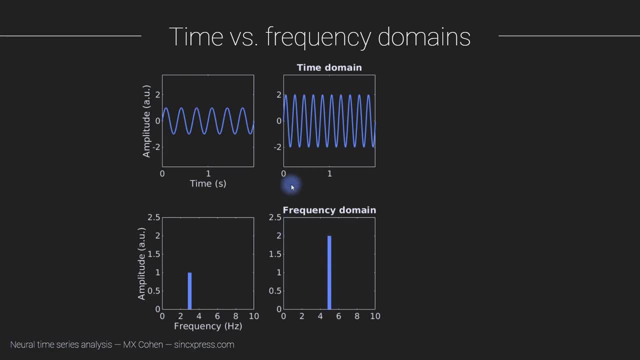 here we see a bar at five Hertz, and then this goes up to two, and here we have the troughs at minus two and the peaks at plus two. That's a total distance of four, and then half of that is two, of course. 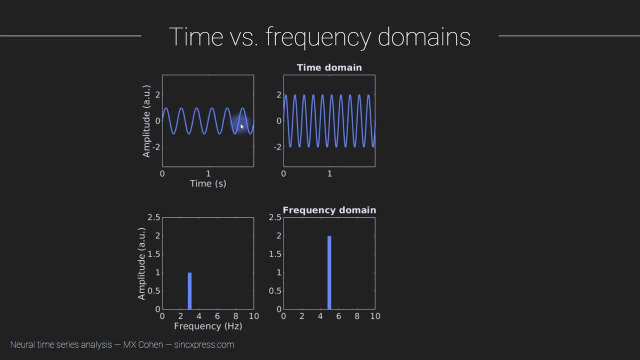 So these are two pretty simple signals. There's really just one component in each of these signals. Here we have another signal which is still pretty simple, but it's a little bit more complicated. It's a little bit more involved. You can probably guess that the way 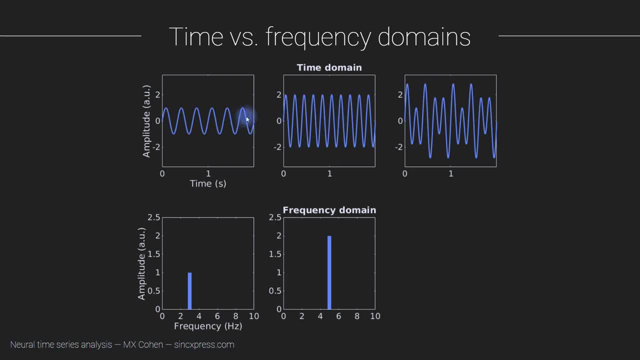 that I created this signal was by combining these two, So literally, this thing plus this thing gives us this thing. Okay, now you know. when you look at this in context, it's pretty easy to tell what's going on. but if I just showed you this signal and asked you, 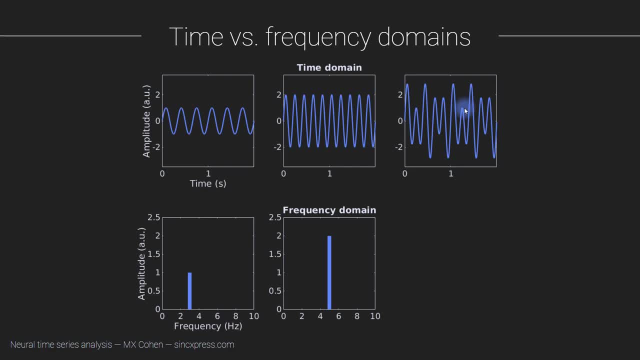 what are the components? how many individual components are there in this signal and what are those components? you could probably figure it out that it was this plus this, but it would take you a little while to figure it out. It would take you. 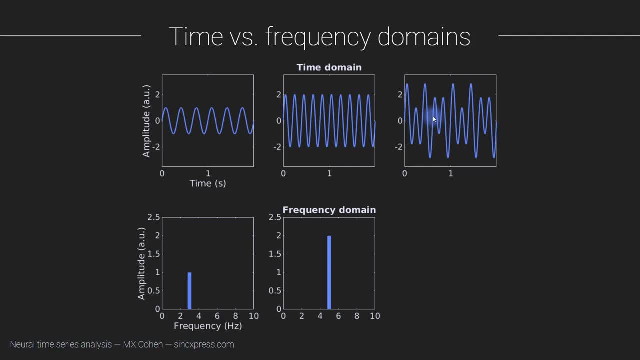 at least several seconds, and that's in the time domain. But now when we go to the frequency domain, it's a totally different story. You look at this signal in the time domain or, sorry, in the frequency domain, and it takes like 50 milliseconds to figure out. 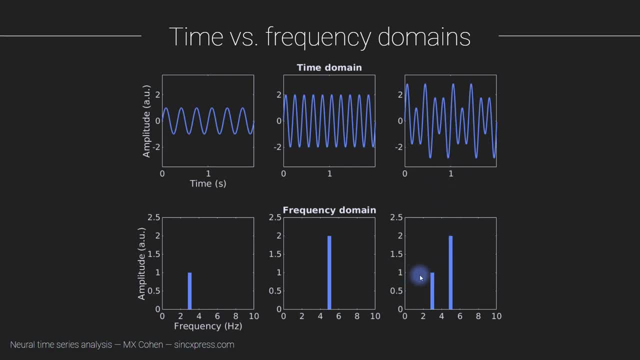 that this signal has two components: one at three hertz with an amplitude of one, and one at five hertz with an amplitude of two. So this, right here, highlights one of the main advantages of looking at a signal and inspecting a signal in the frequency domain. 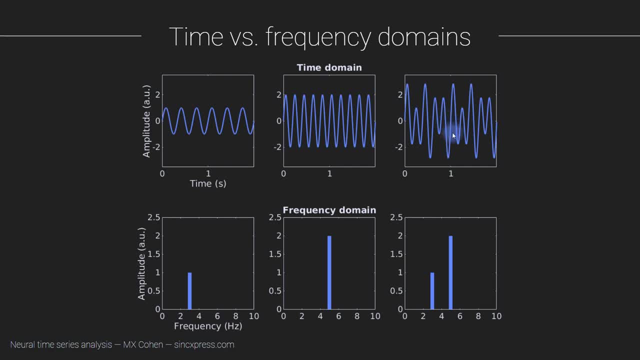 compared to the time domain. And that is that if the signal contains rhythmic narrowband components, which is the case here- it's not the case for all signals- but if the signal is made up of narrowband spectral features, then you can understand the signal much better. 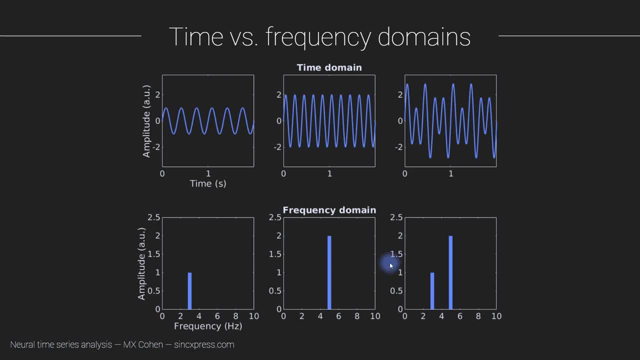 and much faster when looking at the signal in the frequency domain compared to the time domain. Again, that is not trivially true for all signals, regardless of how they're made up. But under some conditions signals are much easier to understand when looking at them in the frequency domain. 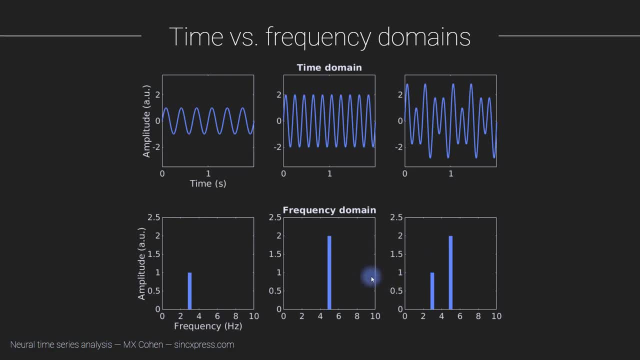 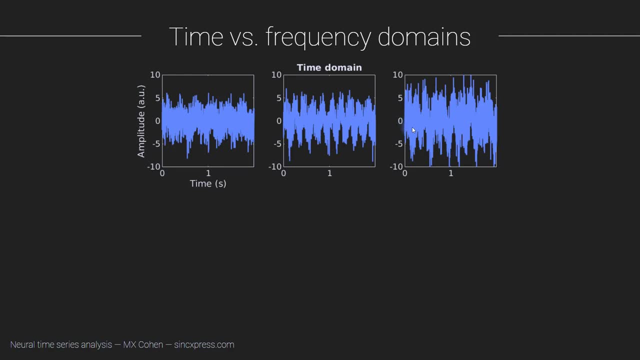 Okay, so that is one advantage of the frequency domain. Now I'm going to show you another advantage, and that is having to do with noise. So here I have exactly the same underlying signals that I showed in the previous slide. The only difference is that I've added randomness. 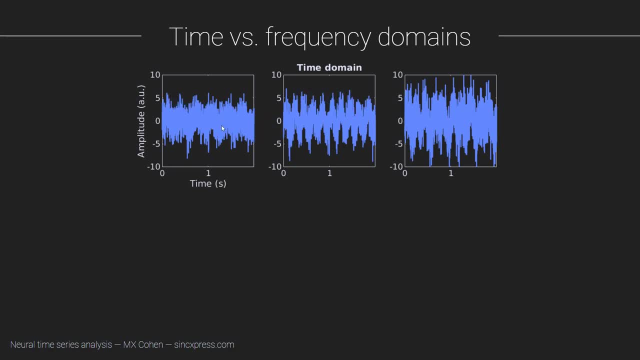 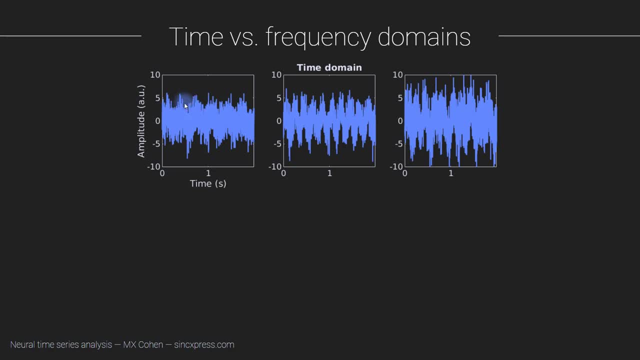 you could figure it out If you looked at this for a few moments. you would say: well, there's one, two, three in one second, and then here it repeats: one, two, three, And here you can count five. 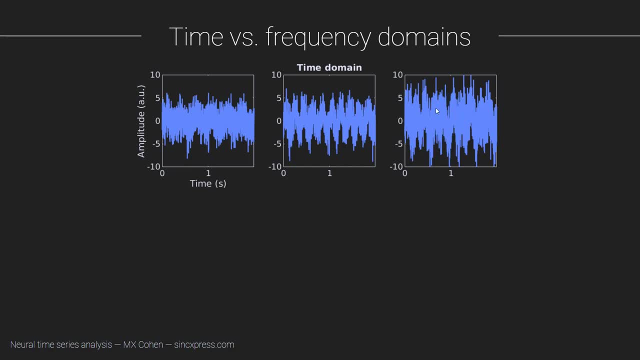 This is going to be much harder. You're not really going to be able to guess that this is a three hertz sine wave plus a five hertz sine wave from looking at this panel. But watch what happens when we go into the frequency domain. 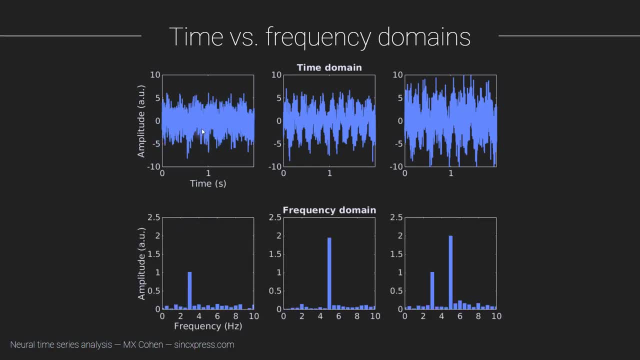 These exact same signals, again with this amount of noise. it's kind of difficult- not impossible, but it's difficult to look at this signal and understand that it's a three hertz signal plus noise. But when you look at it in the frequency domain, 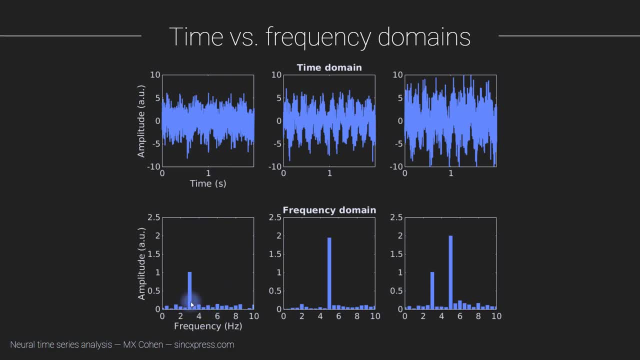 it is totally trivial. You see immediately that we have a three hertz sine wave component with an amplitude of one, plus broadband noise with low amplitude, and same story here and same story here. So the noise is much more deleterious in the time domain. 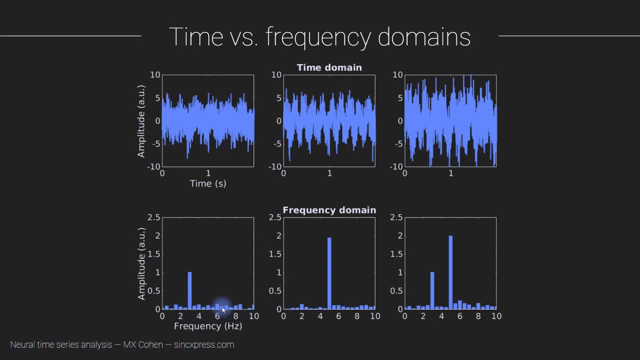 and it's much tinier in the frequency domain. Now, why is that the case? That is happening because this is white noise that I've added. So it has a flat power spectrum in the frequency domain, but the time domain is actually all. 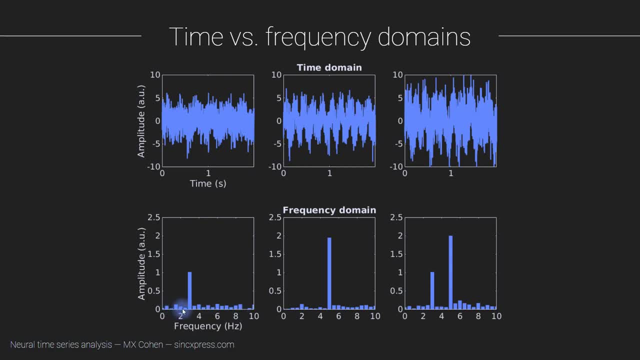 of these frequencies added up. So when you add up all of these little contributions of small power for lots and lots of frequencies in the time domain, that ends up being a large amount of noise, even though for any individual frequency it's quite small. 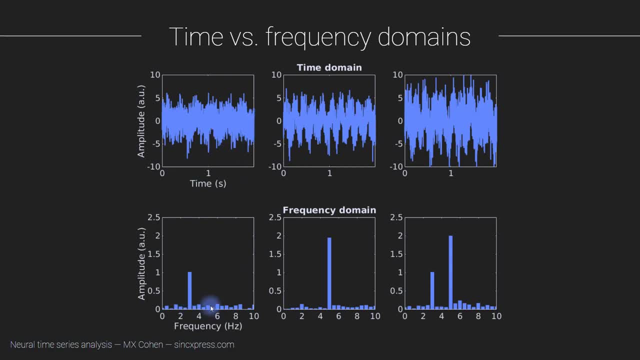 So, therefore, looking at a signal in the frequency domain can also improve the signal-to-noise characteristics of interpreting the signal, And that is the second advantage of the frequency domain, or looking at a signal in the frequency domain, that I would like to highlight in this video. 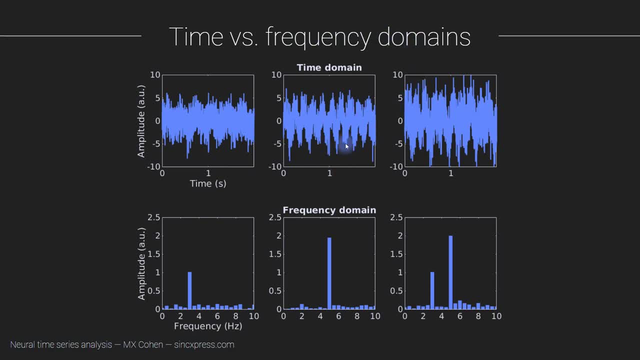 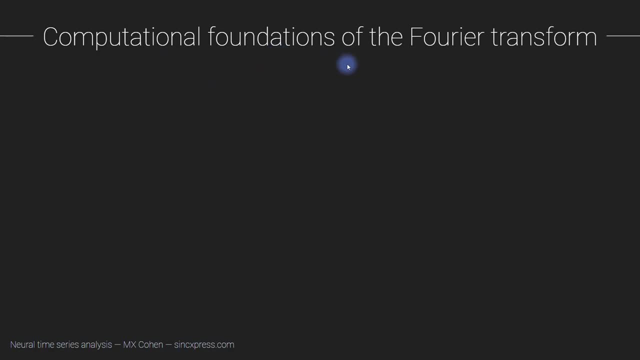 Okay, so that's all I'm gonna say about time and frequency domains for now. And then I want to mention briefly the computational foundations of the Fourier transform. So what I'm going to show you in this slide is a diagram of all the individual things, the pieces of knowledge. 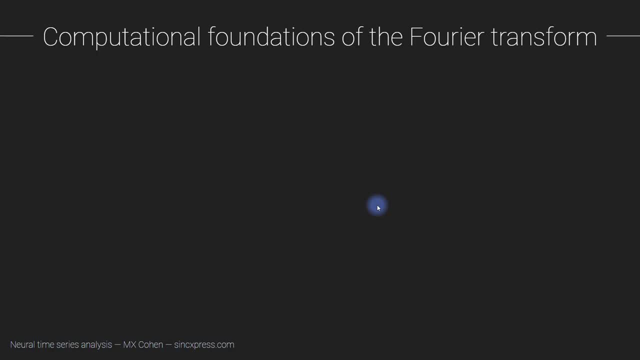 that you need to acquire in order to completely understand the Fourier transform, the discrete Fourier transform. So we start with the most important foundational parts and that's these three things here. So you need to know about sine waves, you need to know about complex numbers. 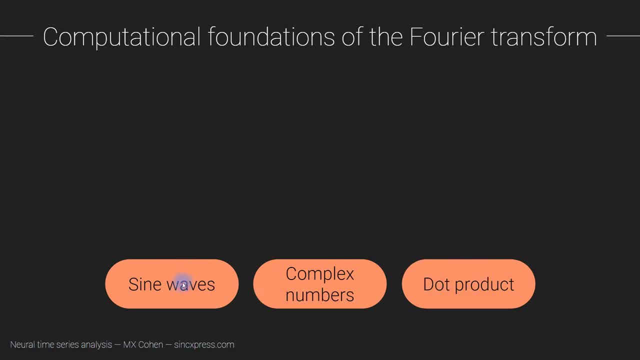 and you need to know about the Dop product. Now, I'm sure you've heard about sine waves, You've probably heard about complex numbers, but maybe you haven't- And maybe some of you have- heard of the Dop product, or maybe you haven't really heard of the Dop product. 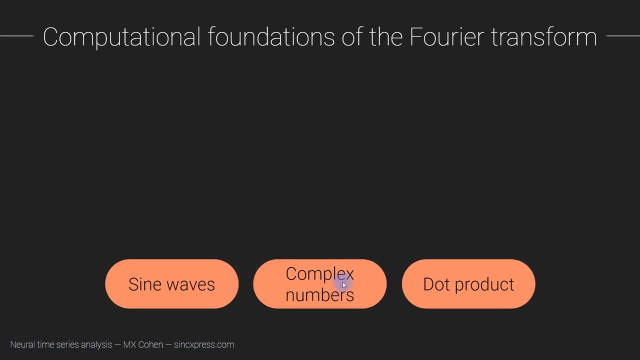 So, regardless of how familiar you are with these three concepts, I'm going to show you a little bit. So we'll start with the first one. We'll start with the second one. We'll start with the first one, So we'll start with the second one.